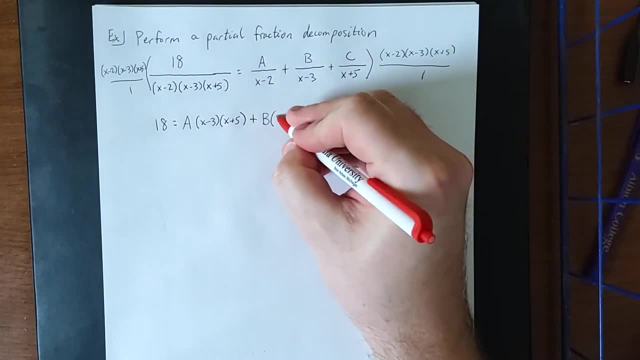 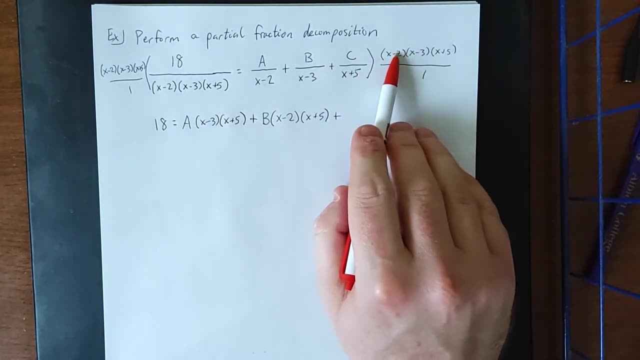 The two things left attached to b will be x minus 2 and x plus 5.. Same thing will happen on the c term. We distribute all three of these to this term. The x minus 5 will cancel with the x minus 5.. 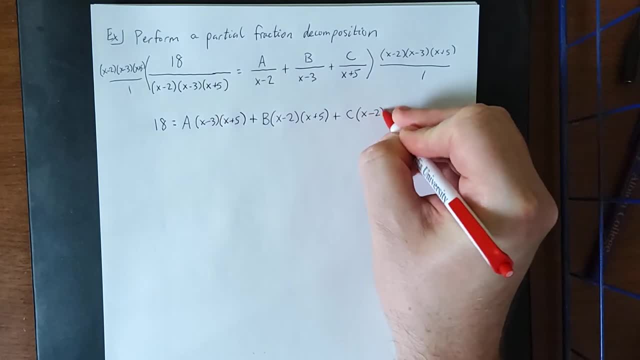 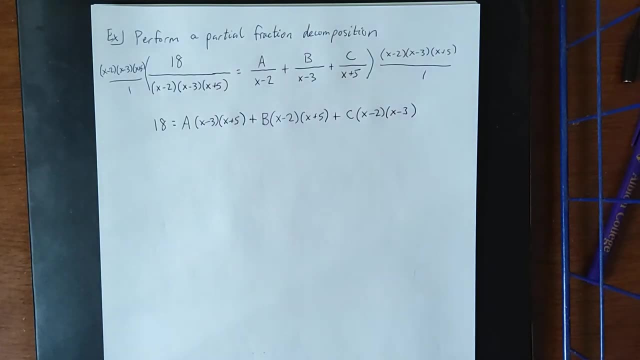 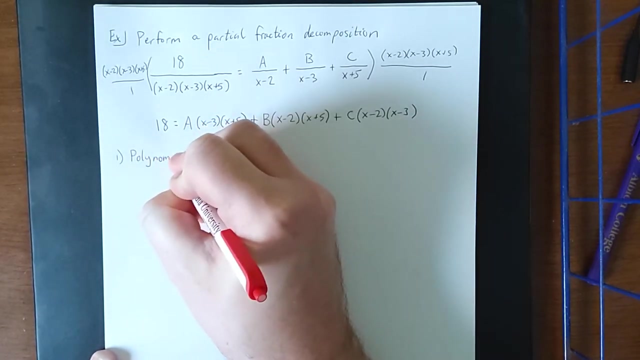 And we will be left with c times x minus 2 times x minus 3.. Now there are two methods for how to proceed from here, and I'm going to be demonstrating both of them. The first one is that we can set up that a polynomial is equal to a polynomial. 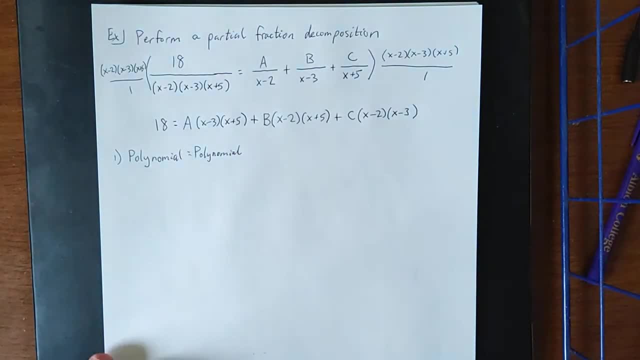 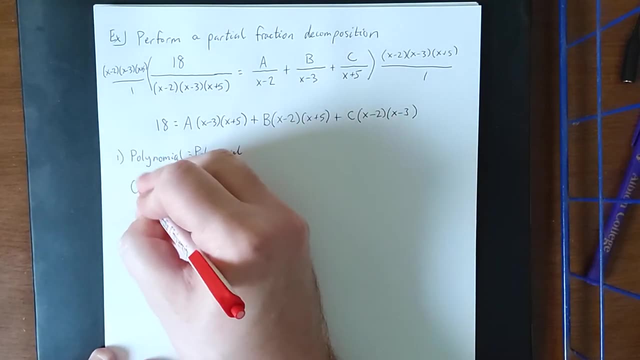 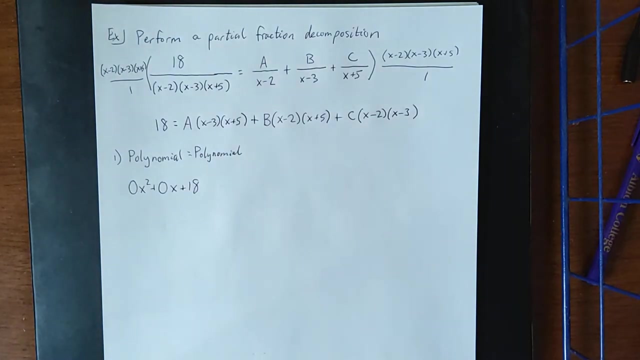 Now on the right-hand side. once this thing is expanded completely, we are going to wind up with a quadratic polynomial on the right-hand side. So I'm also going to express the left-hand side as a quadratic polynomial. However, given that it has no quadratic term and no linear term, 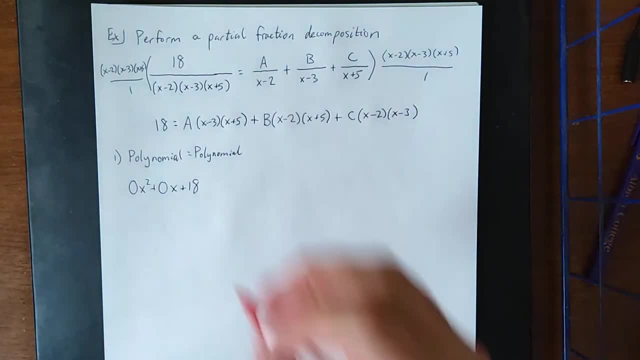 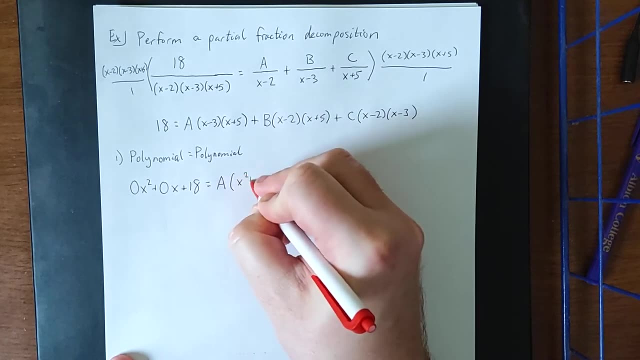 we're going to be using a quadratic polynomial, So I'm going to call this 0x squared plus 0x plus 18.. To expand the right-hand side, I'm going to be using my second favorite four-letter f-word, That is, FOIL. 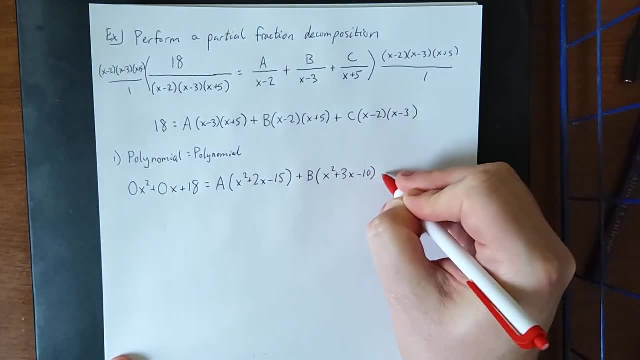 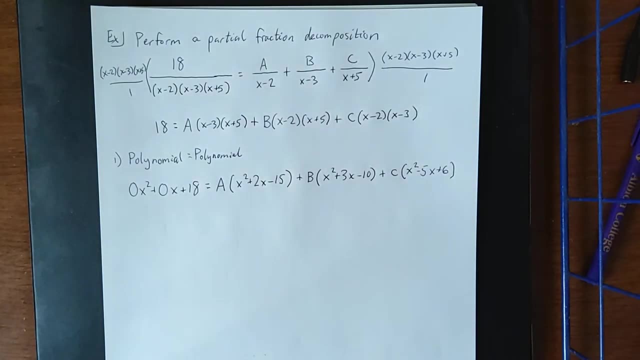 So in all of the cases where we have a linear factor times a linear factor, we're going to go ahead and FOIL those out. Then we can distribute the a, b and the c, But ultimately we're going to be using a quadratic polynomial. 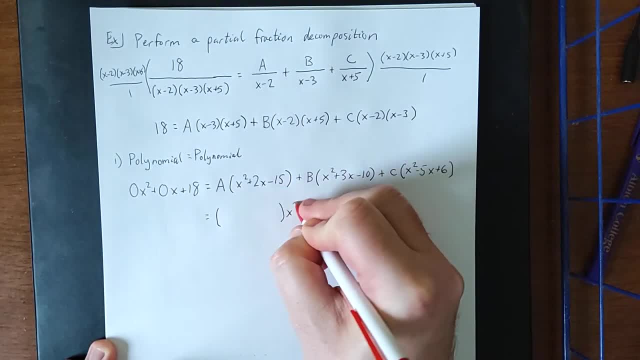 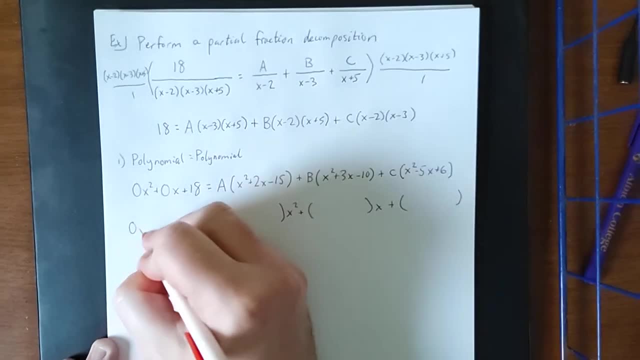 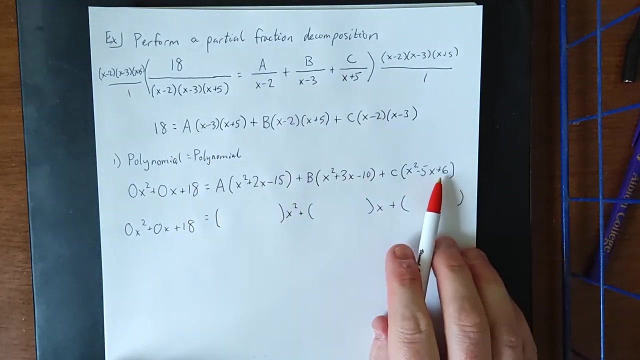 And ultimately, what we're trying to end up with is some coefficient times x squared plus some coefficient times x plus some constant term. Now, if we take a look through at all of the x squared terms that we're going to get through here, we are going to get an ax squared plus bx squared plus cx squared. 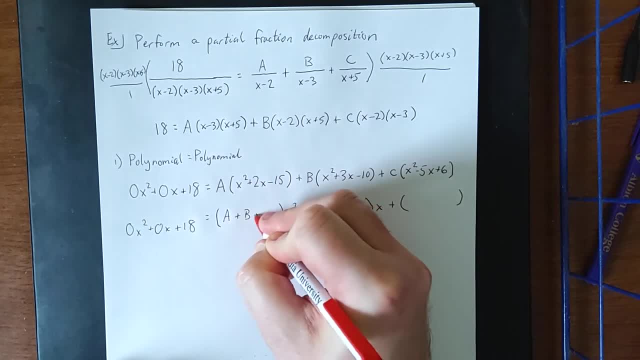 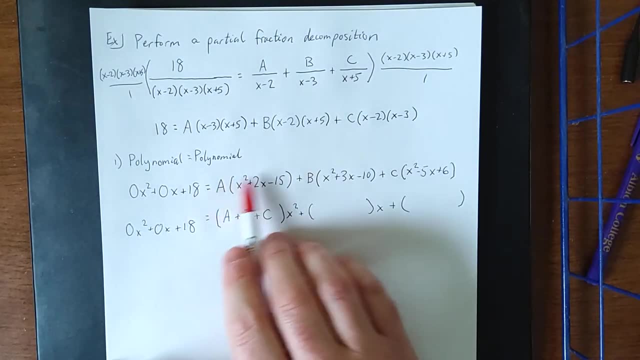 If we factor out the x squared, that's going to leave us with a plus b plus c. If we take a look at all of the x terms, we are going to wind up with 2ax plus 3bx minus 5cx. 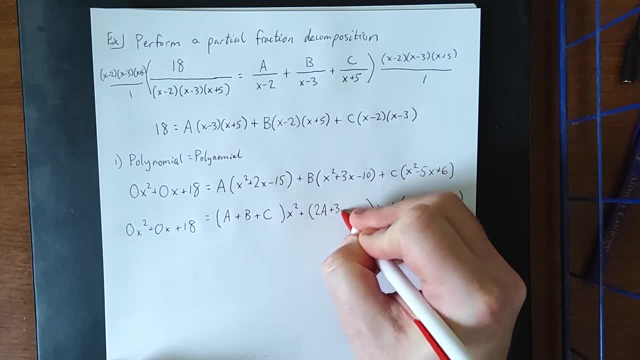 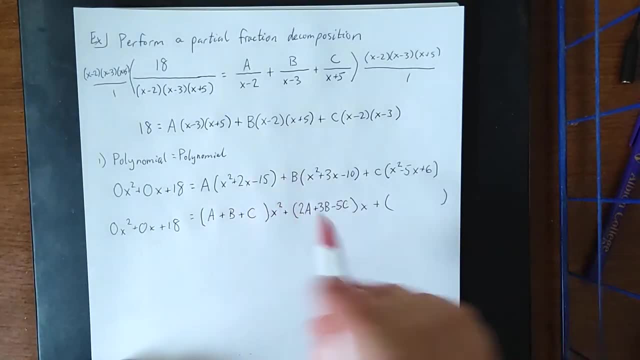 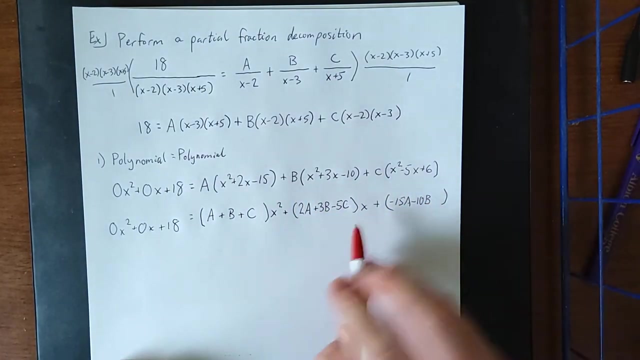 Factoring out the x from each of those terms would be 2a plus 3b minus 5c And finally, the terms without x's. we are going to see a negative 15a minus 10b plus 10b plus 9b plus 12b plus 10b plus 15b plus 16b plus eight. 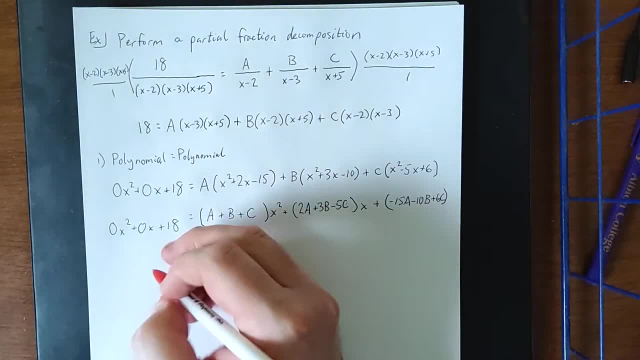 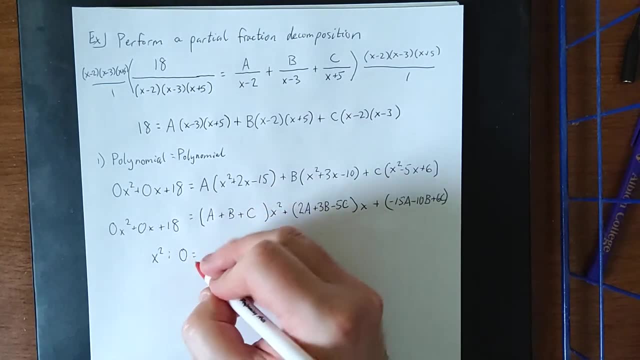 Now the way that this means that polynomial is equal to polynomial is that the corresponding coefficients of corresponding powers of x will be equal to one another. That allows us to conclude that the coefficients of x squared will be equal. On the left hand side, that would be simply zero. 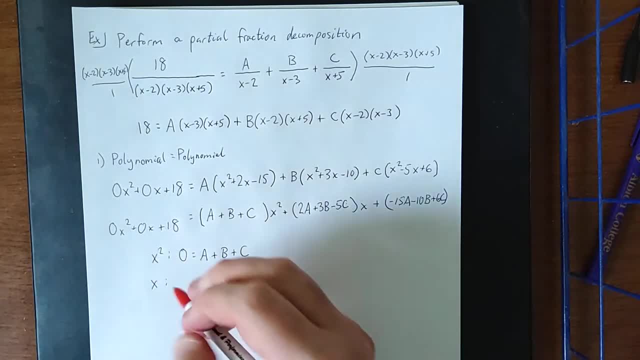 will be equal as well. On the left hand side, the coefficient of x is simply 0.. On the right hand side, the coefficient of x is 2a plus 3b minus 5c. On the left hand side, the constant term. 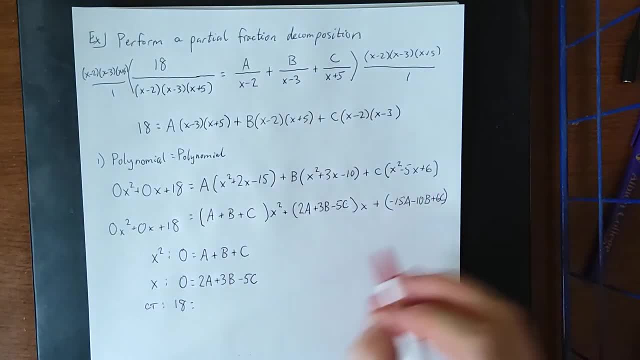 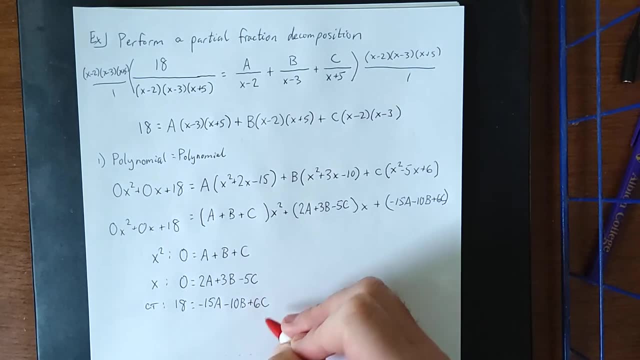 is 18.. On the right hand side, the constant term is negative: 15a minus 10b plus 6c. At this point, what you're left with is a system of three equations with three variables, which you are now welcome to solve for a, b and c. Now what I'm going to do to solve for a, b and c. 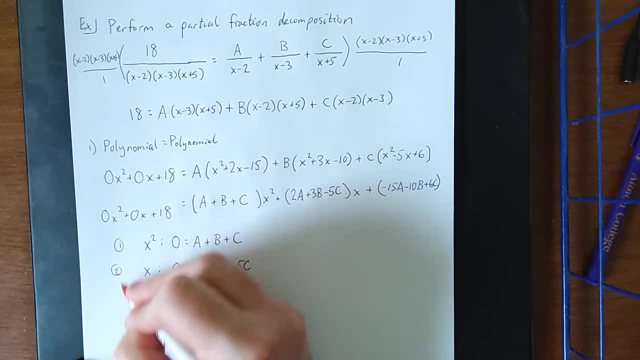 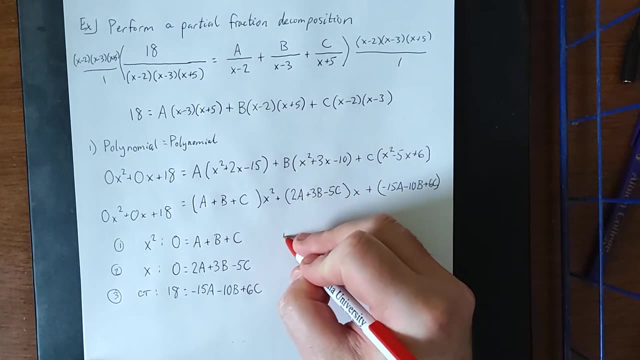 is. I'm going to label these as equation number one, number two and number three. First thing I'd like to do is eliminate all of the a terms to leave me with just b and c. I'm going to take 15 times equation number one and add it to. 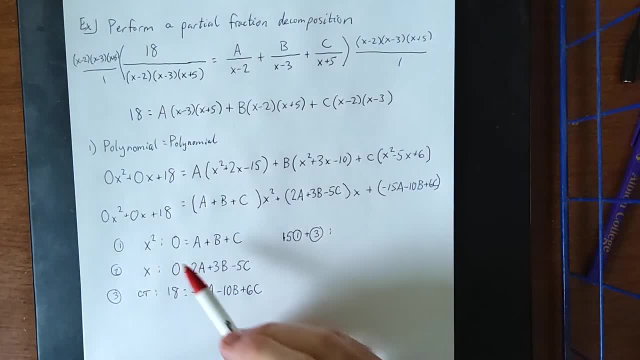 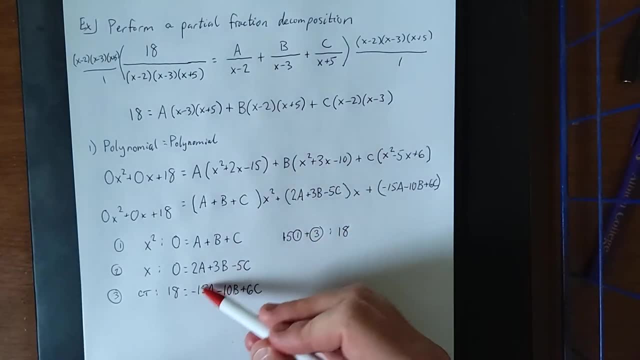 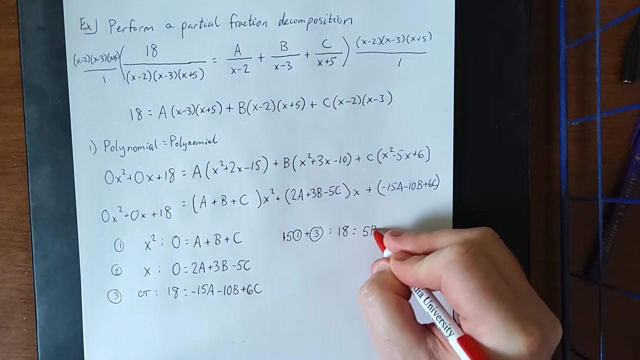 equation number three. So I'm going to take 15 times 0, add it to 18.. I'm going to take 15 times a and add it to negative-15a, which will eliminate my a variable. 15 times b, add it to negative-10b, That'll be positive-5b. 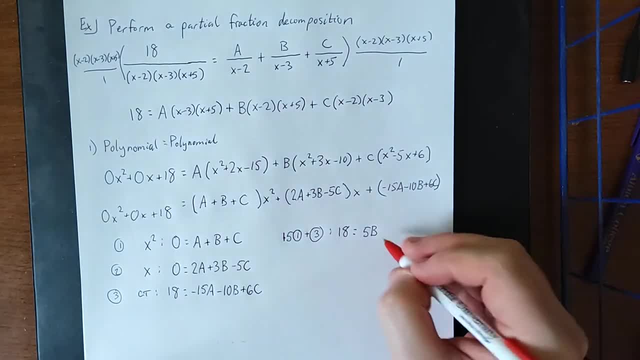 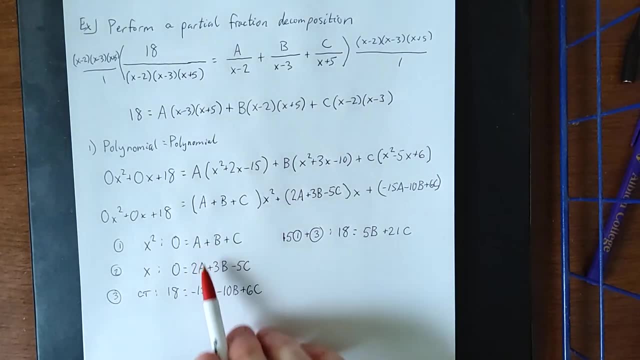 Then I'm going to take 15 times c and add it to 6c, for a total of 21c. To further eliminate the a variable, take the whole two. Now, with that all done, I'm going to take the whole Cohen Okay, le wide conduct example and then roughlyży me the sum of the winnings. 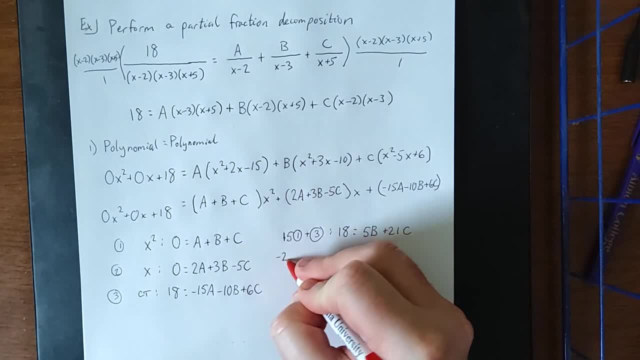 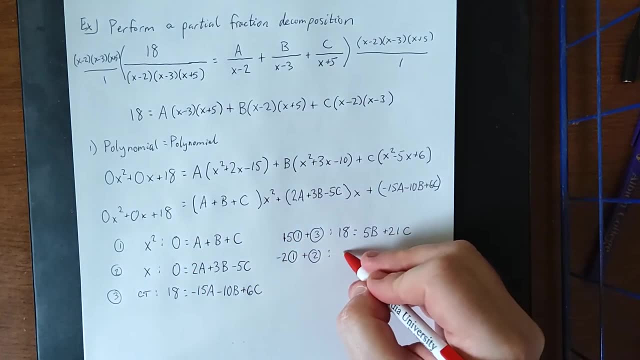 I'm going to use the first two equations, So I'll take negative 2 times equation number 1.. I'm going to add it to equation number 2.. So negative 2 times 0 added to 0 will be 0.. Negative 2 times a added to positive 2a: that is where an 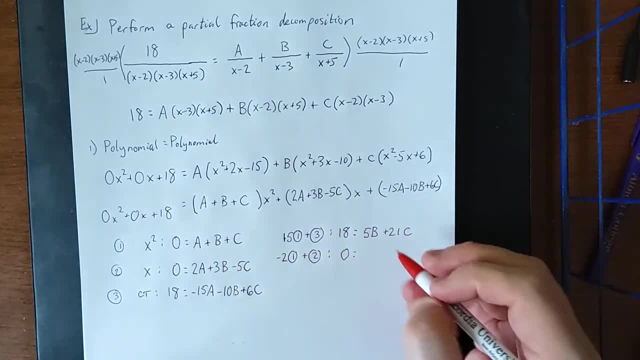 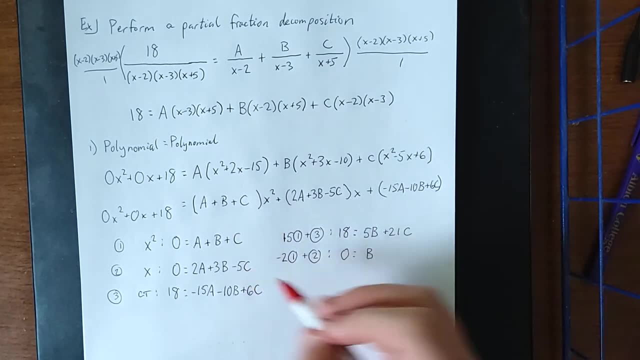 elimination will take place. Negative 2 times b added to 3b will be simply b. Then negative 2 times c added to negative 5c will be negative 7c. We're looking good so far. Next, from these two equations that I have here, I think I'd 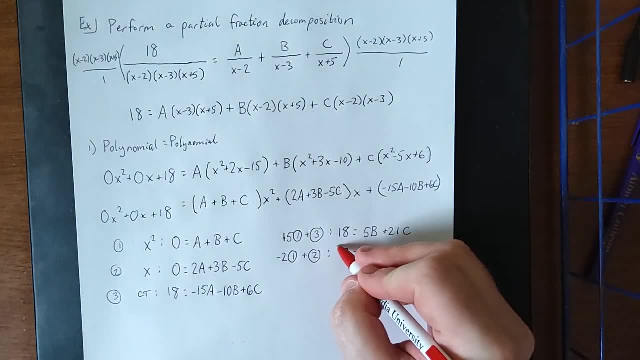 like to eliminate the c variable, since it's already in pretty good shape to do so. I'm going to take the second equation that I just got, multiply it by 3, and then add these two equations together. So 18 plus 3 times 0 is 18.. 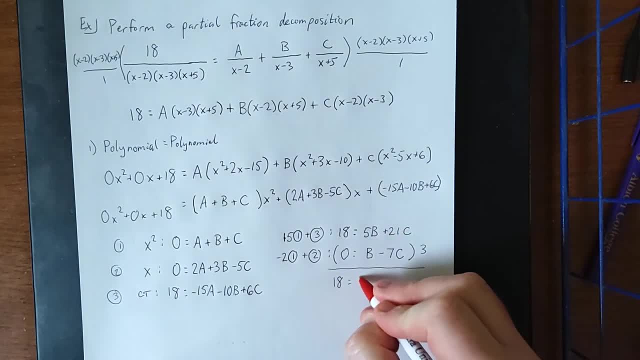 So 18 plus 3 times 0 is 18.. So 18 plus 3 times 0 is 18.. 5b plus 3 times b is 8b, And then 21c plus negative 21c. those will eliminate. 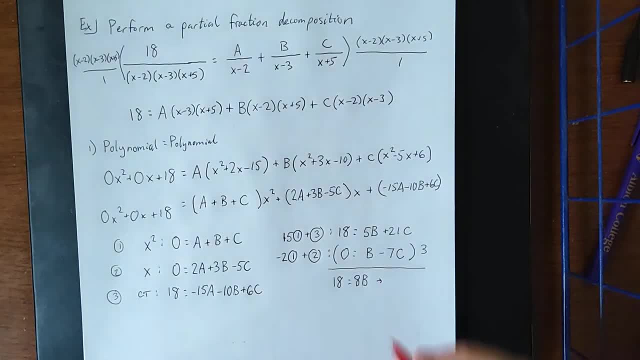 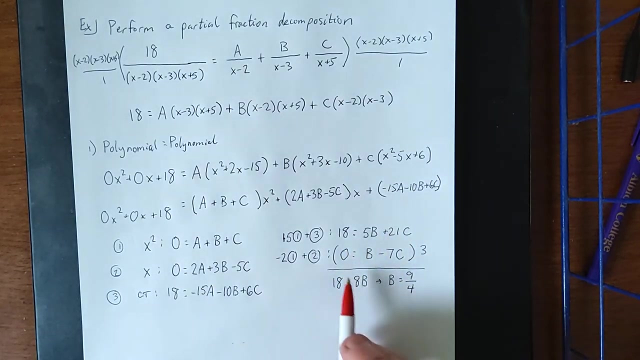 completely. We're left with: 8b is equal to 18.. Solving for b can be done by dividing both sides by 8, reducing down to 9 fourths. Then I can take this value for b and plug it into either of these equations. to solve for c Now this: 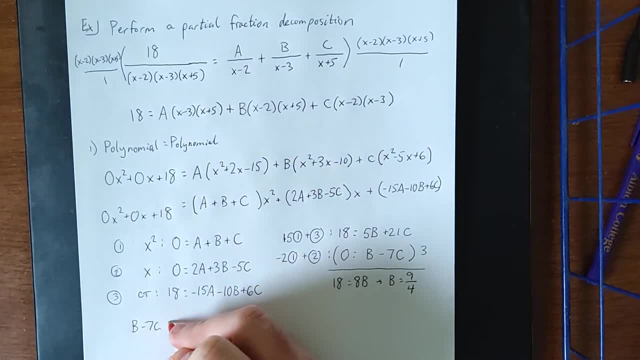 equation right here is going to be the same as the equation for b. I'm going to plug it into either of these equations to solve for c. Now, the value of the value of b, which was b minus 7c, is equal to 0, is equivalent to saying that b is equal. 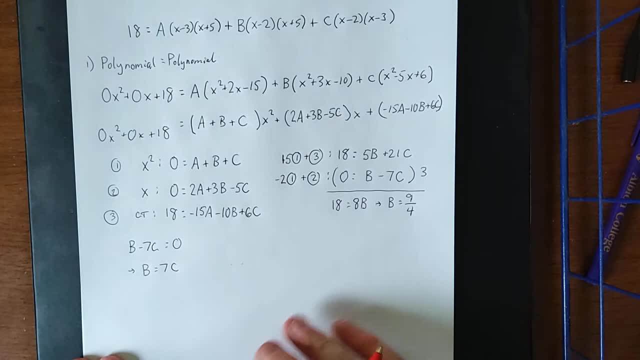 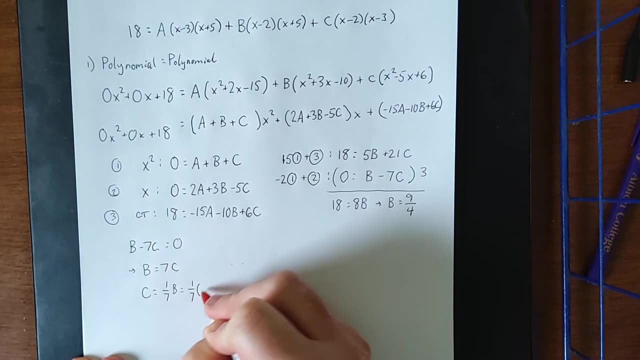 to 7c Now, because we have the value of b. I'm going to solve this for c and say that c is equal to one seventh of b, or one-seventh of nine fourths, therefore telling us that this would be 9 over 28.. Now equation number one tells me that a: 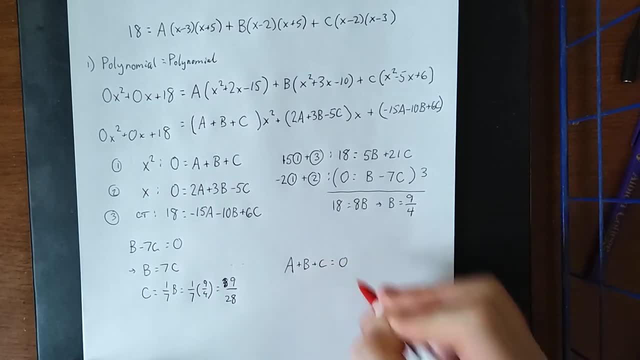 plus b plus c was equal to 0, also telling me that a would be equal to negative b minus c. So we'll take negative 9 fourths and subtract 9- twenty-eighths. Get a common denominator for this by multiplying the first. 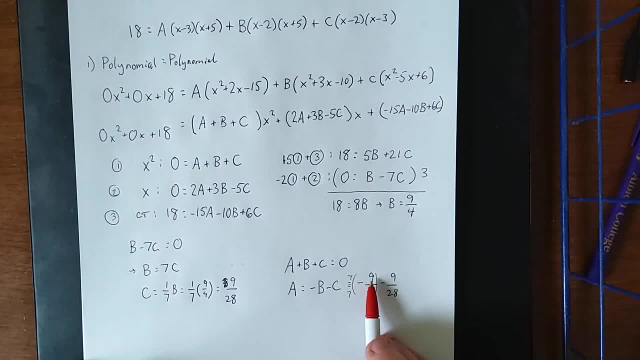 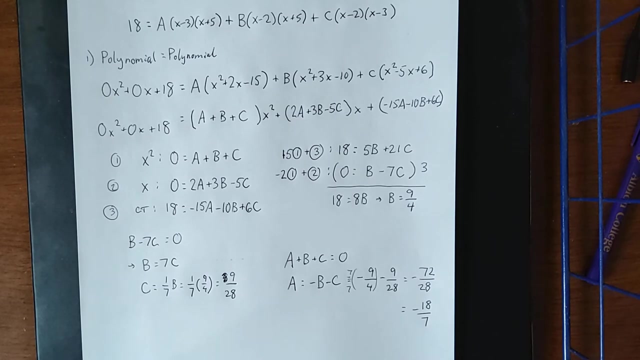 fraction by 7 over 7.. This will be at negative 63 minus 9,, which will be negative 72 over 28.. Reducing this fraction as much as possible gives us negative 18 over 7.. Now, this is the technique of polynomial equals. 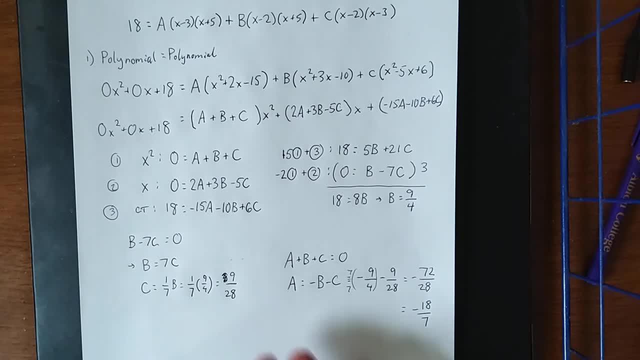 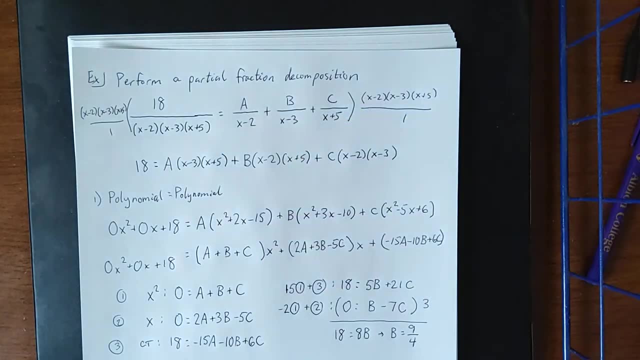 polynomial and it can always work. The problem is that if you start with a degree of n, you are going to be setting up a system of n equations with n variables. So once you get up to a degree four or a degree five, polynomial. well, 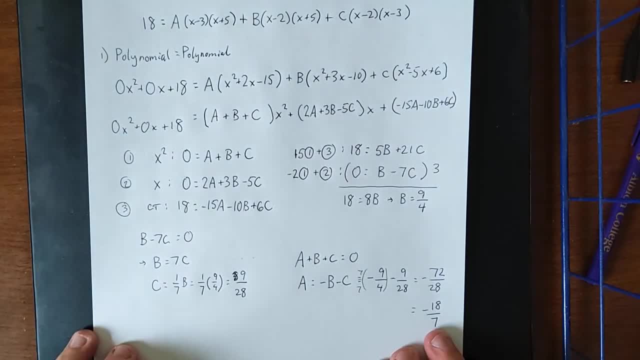 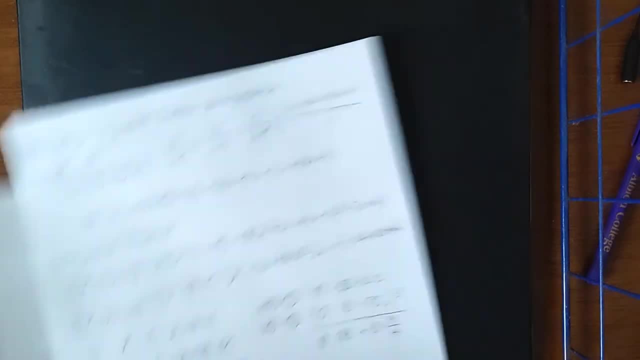 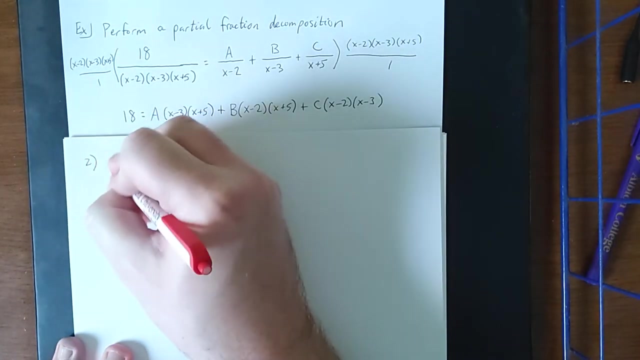 you're looking for a lot of substitution that you wouldn't want to necessarily do So instead, I'd like to demonstrate the other technique for how we could potentially solve something like this. So, with that in mind, the second technique works especially well if all that you have is linear factors. I 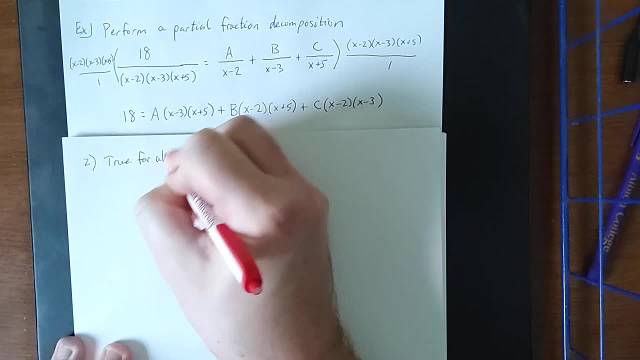 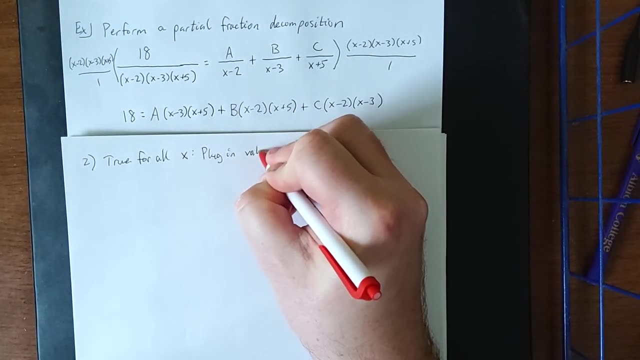 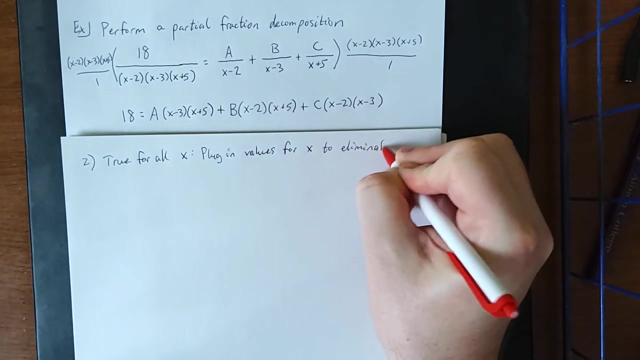 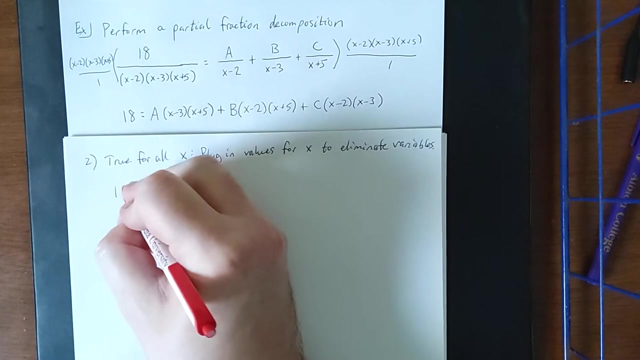 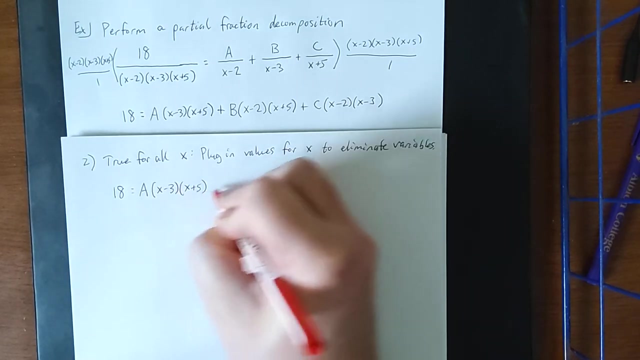 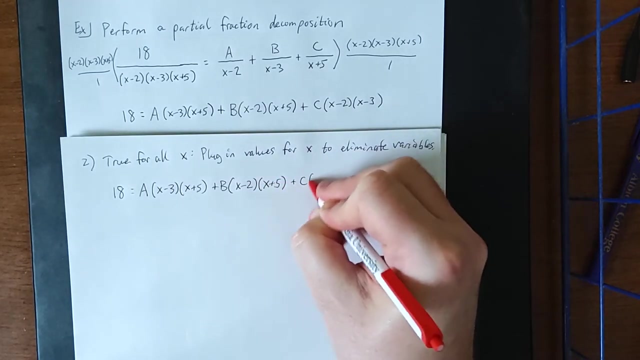 refer to this one as true for all x. The strategy is we are going to plug in values for X to eliminate variables. By variables I'm referring to a, b and c. So once again, 18 is equal to a times x minus 3, times x plus 5, plus b, times x minus 2, times x plus 5, plus c. 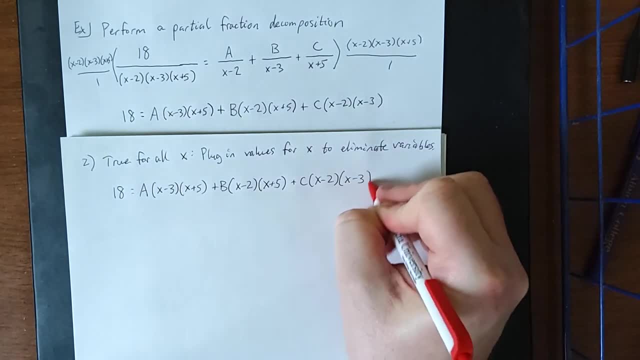 times t minus 2.. So that should go Hurry, hurry, hurry. Okay, that's your first principle. And then that would indeed help if our next proposal could be long, short or pistol-shooting: x minus 2 times x minus 3.. So again, we are trying to plug in values of x to eliminate some of the 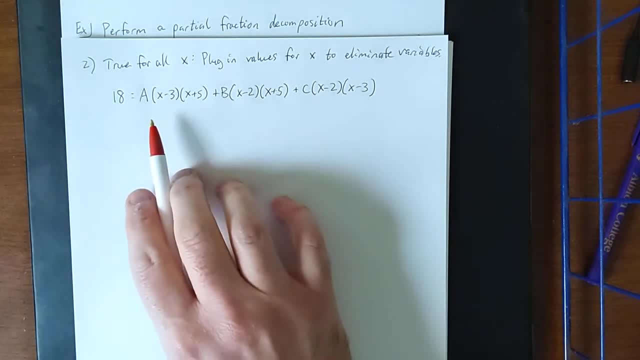 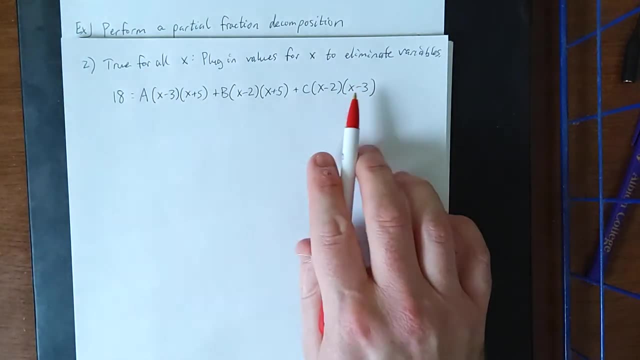 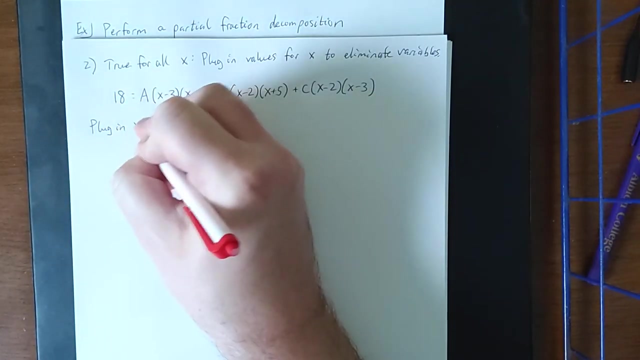 variables that we have present. So I notice that there's an x minus 3 in two of the terms here. Now what would I plug in for x? to turn x minus 3 to 0?? I'm going to plug in: x is equal to 3.. 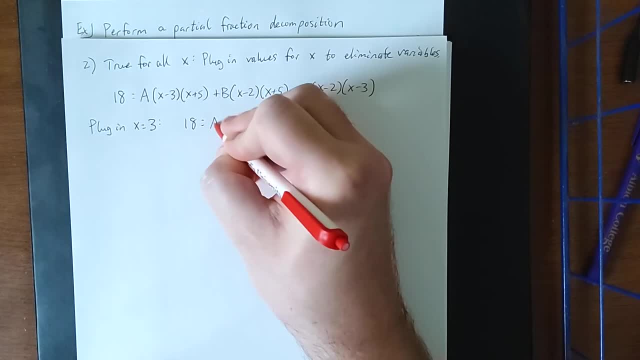 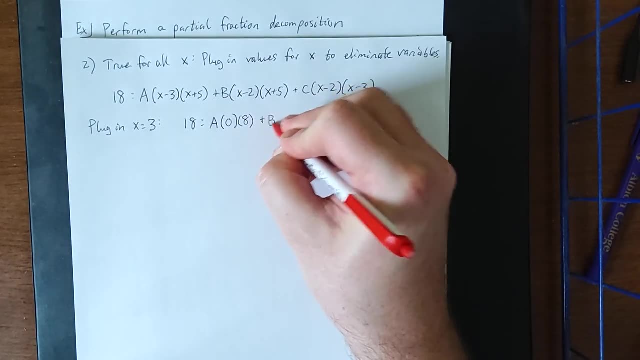 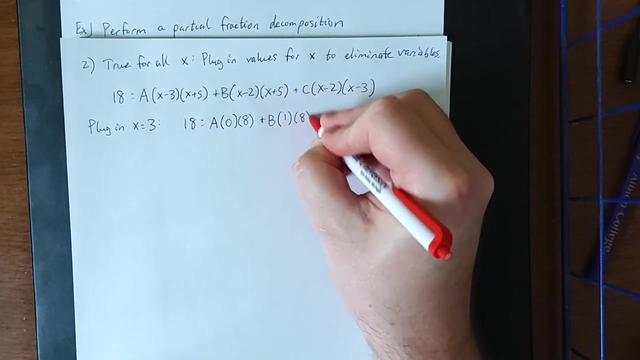 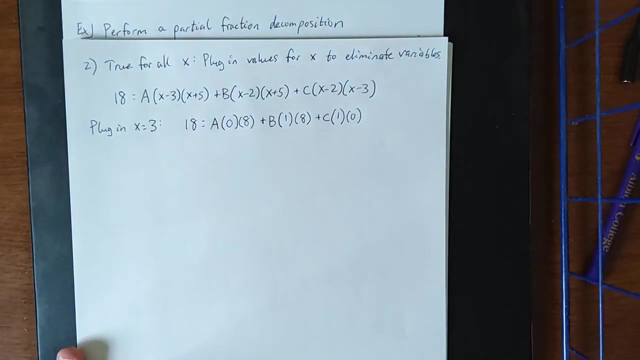 That would give us, once we plug it in 18, is equal to a times 3 minus 3 times 3 plus 5 plus b times 3 minus 2 times 3 plus 5 plus c times 3 minus 2 times 3 minus 3.. What we're left with after all of these? 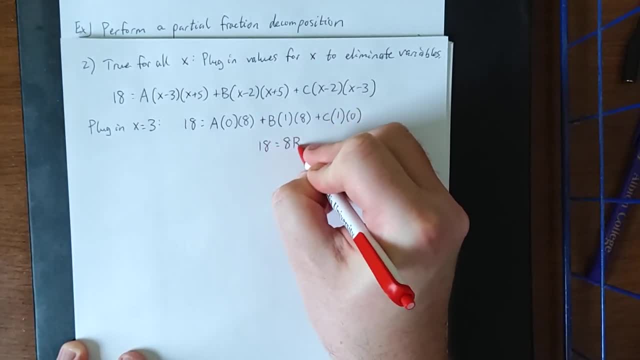 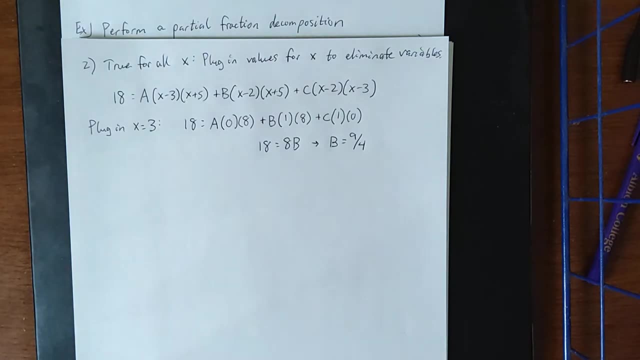 shenanigans ensue- is 18 is equal to 8.. Telling us that b is equal to 18 over 8, which reduces to 9 over 4, same as what we got using the previous method. Now, if I'm interested in solving for b, nope, just did that. If I'm. 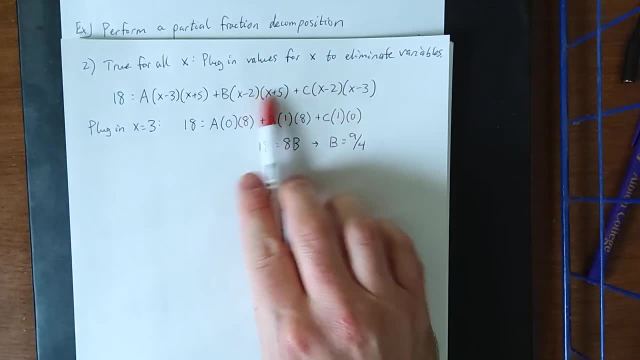 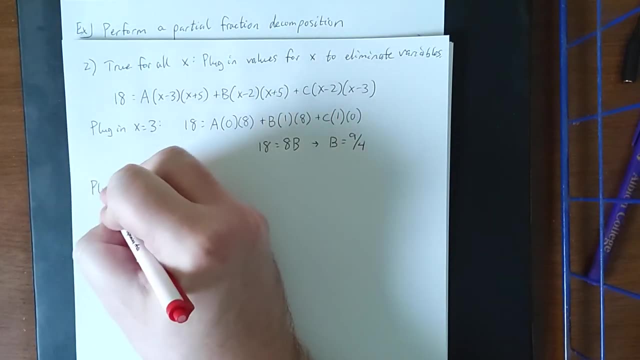 interested in solving for a the two factors that b and c have in common. they both have an x minus 2.. What I'd like to do is plug in something to turn x minus 2 equal to 0. So I'm going to plug. 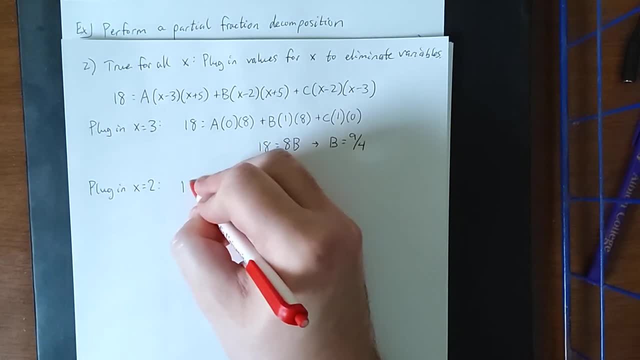 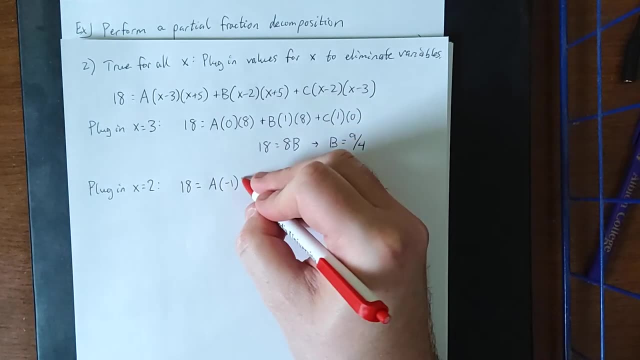 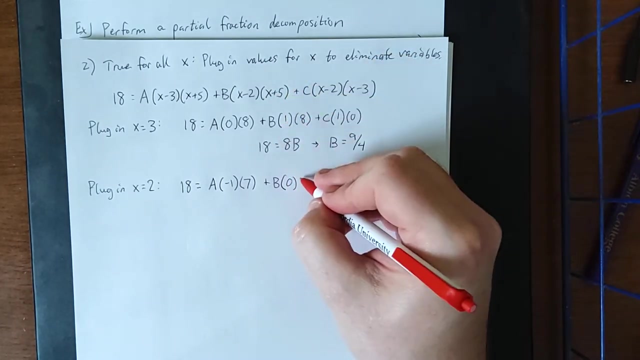 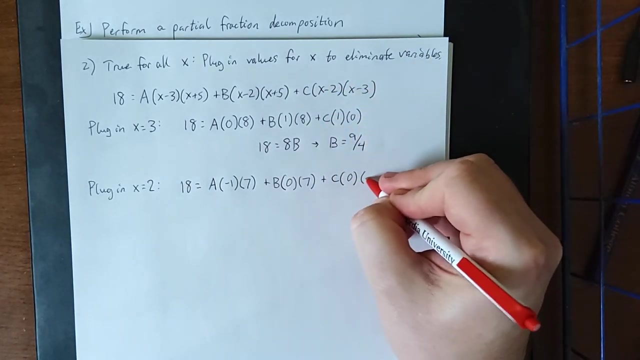 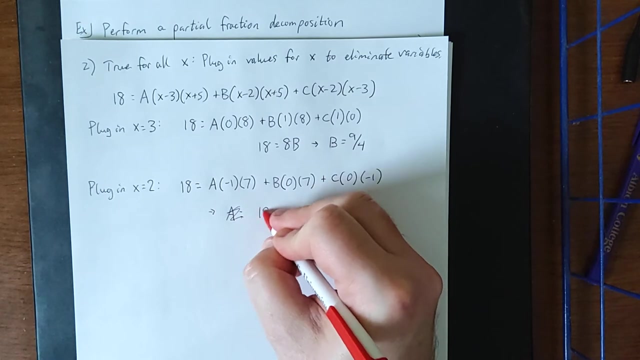 in x is equal to 2.. Giving me 18 is equal to a times 2 minus 3 times 2 plus 5 plus b times 2 minus 2 times 2 plus 5 plus c times 2 minus 2 times 2 minus 3.. Leaving me with a is equal to- oh, excuse me, 18 is equal to. 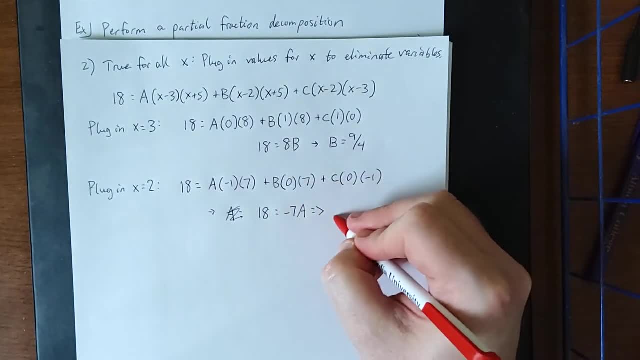 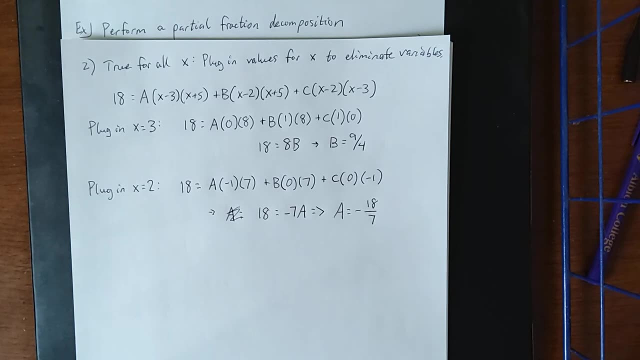 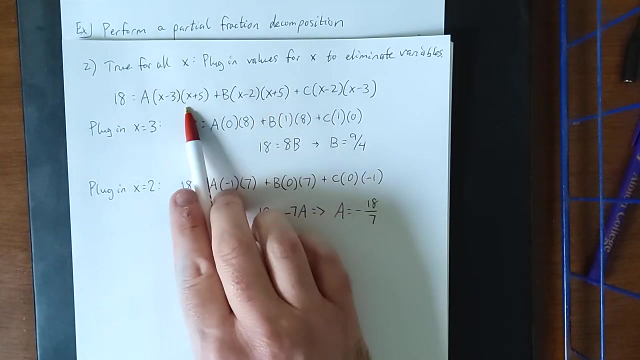 negative 7a, Telling me that a is equal to negative 18 sevenths. Finally, if I'm interested in solving for c, I would want to plug in something to cancel out the a and b terms. Now they both have a factor of x plus 5 associated with that. so what I'm going to do is plug in x equals whatever. 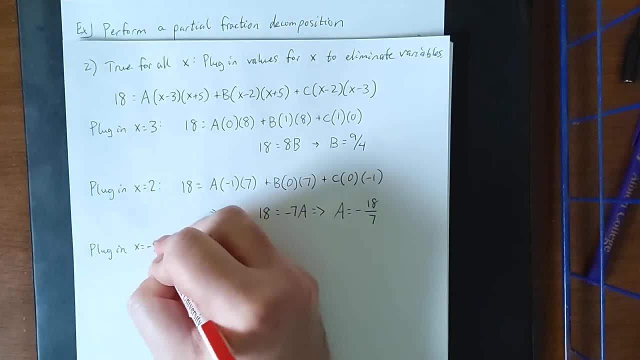 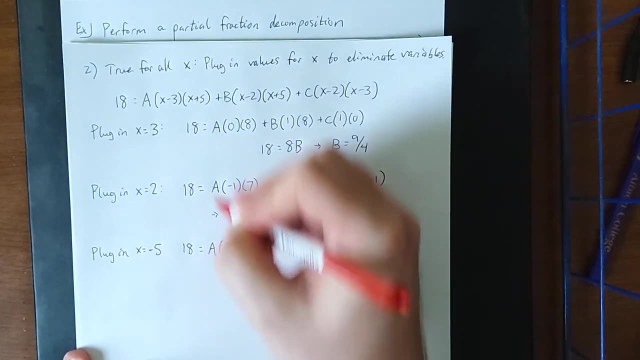 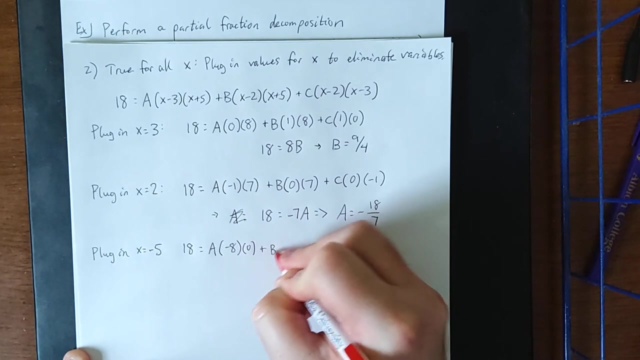 value is going to turn x plus 5 equal to 0.. Well, that would be: x is equal to negative 5.. We wind up with: 18 is equal to a times negative, 5 minus 3 times negative 5 plus 5 plus b times. 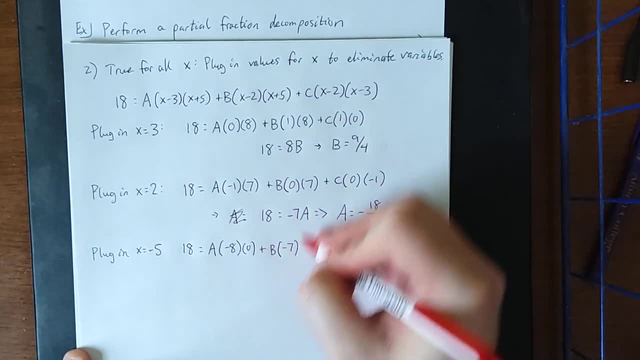 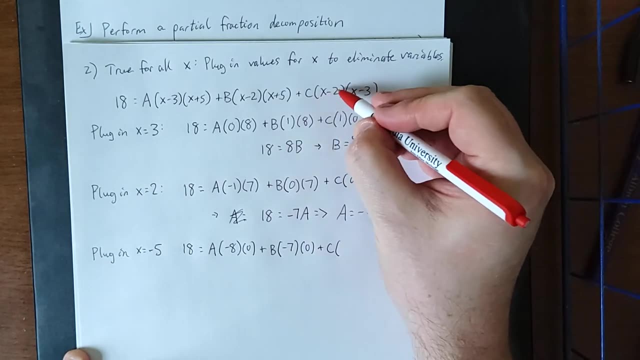 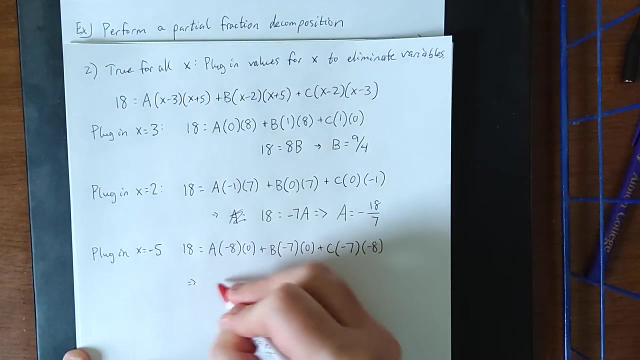 negative 5 minus 2 times negative 5 minus- excuse me, negative 5 plus 5 plus c times negative 5 minus 2 and negative 5 minus 3.. This results in 18 is equal to negative 7 times negative 8, which is 56 times c dividing both. 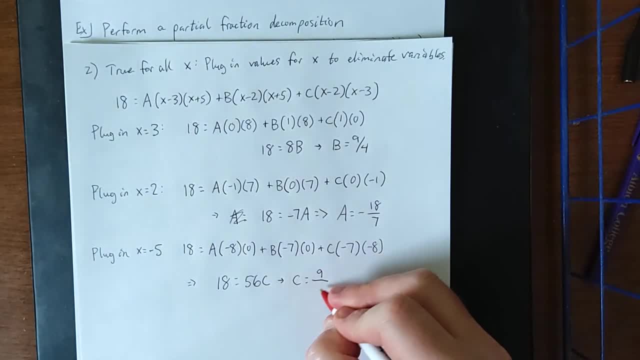 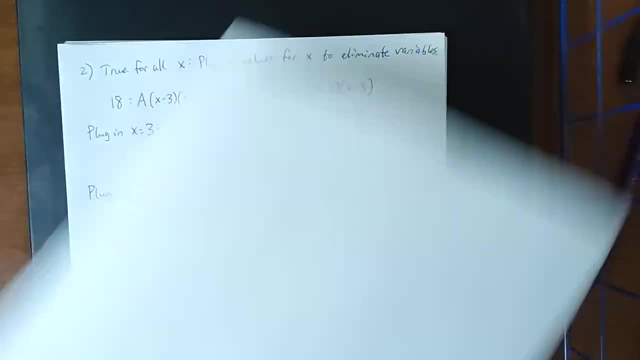 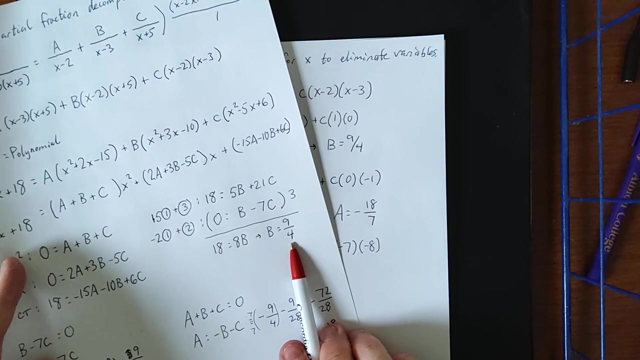 sides by 56 and reducing by a factor of 2 will give us 9 over 28.. Now when we compare that to the results on the previous page, we got b is equal to 9 fourths, which is what we got on the.